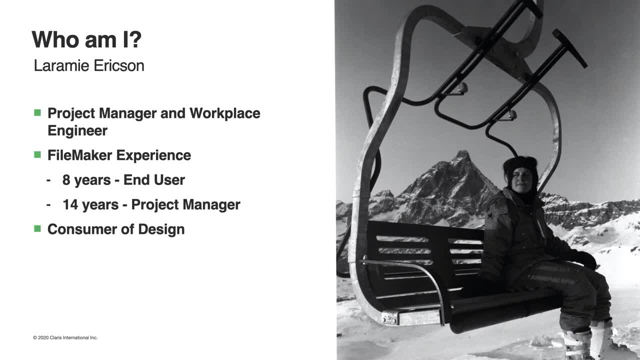 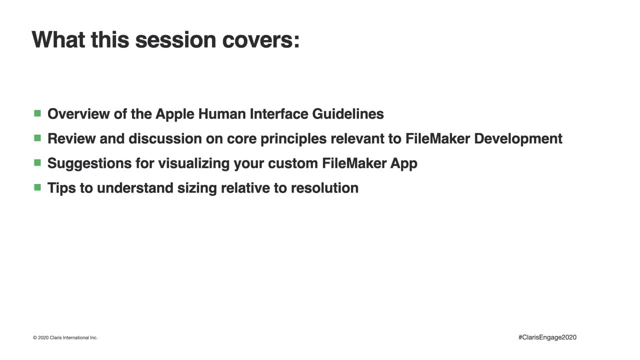 of beauty and simplicity- Mostly toys, but that's for another day. In this session we'll cover an overview of the Apple iOS Human Interface Guidelines. We'll have time to review some of the core principles that I believe are relevant to FileMaker design and development And looking at suggestions for visualizing. 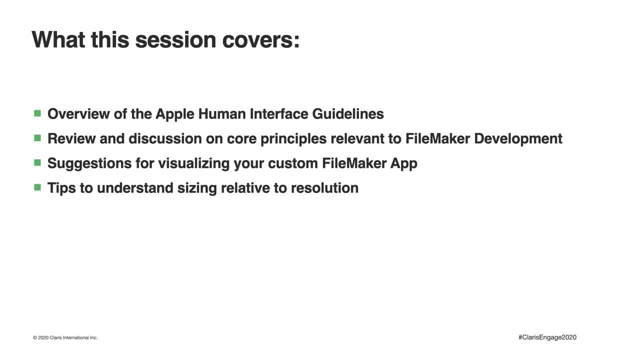 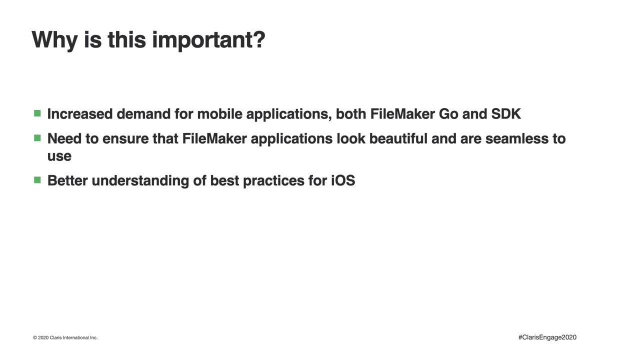 the application, how do you bring it about, How do you plan it. And then also I'll go into a couple of little tips that I've learned along the way about understanding, sizing and resolution, Design and Love. So you might ask, why do we want to do this? And my pure answer is that we are constantly. 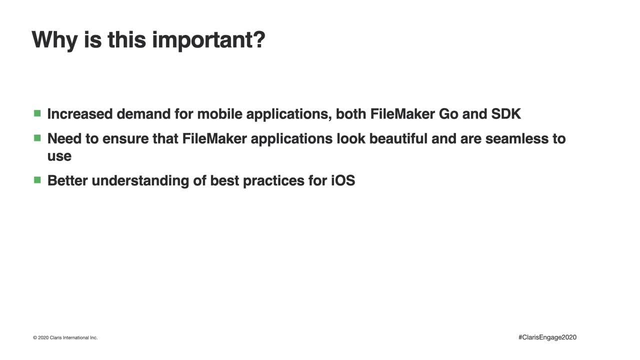 seeing an increase in requests for mobile applications. People will especially look, want to have. people want to use FileMaker Go. they want to have applications built for their iPhone. they want to have applications built for their iPads. they have business uses where their employees could accomplish. 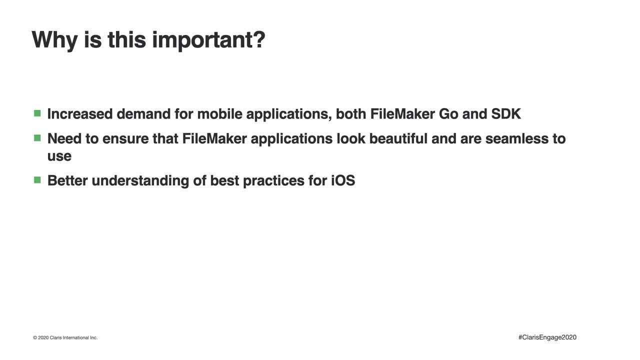 simple tasks if they had a device that was out in the field with them. they as managers or as business owners, have needs where they would find it useful to have to be able to pull out their phone and to be able to accomplish some of their business purposes there, and because of that we need to make sure. 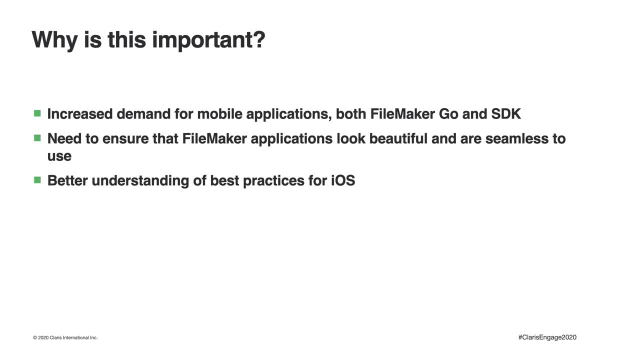 that our FileMaker applications are beautiful and they are seamless to use, because now we are, we're introducing this aspect of designing onto a phone and as we and as we go further into our design practices and our best practices, we need to make sure that we are able to deliver a product in a way that they 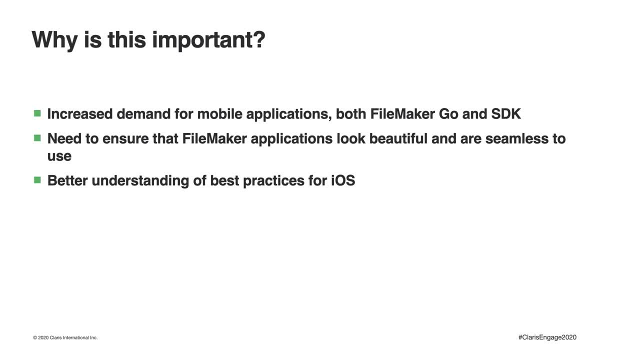 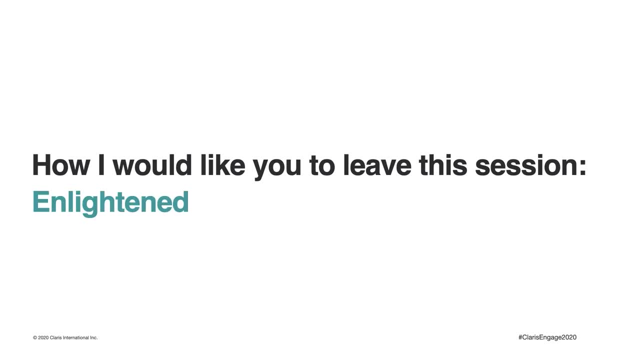 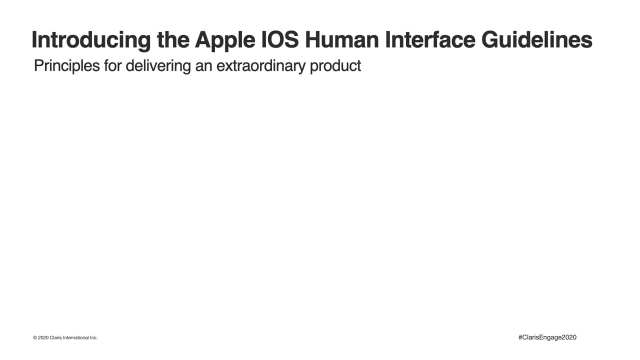 need to also incorporate. what are those best practices for iOS? I would like you to leave this session enlightened. In this chapter, I'll be introducing the Apple iOS Human Interface Guidelines. These are key principles for what is used for delivering an extraordinary product. 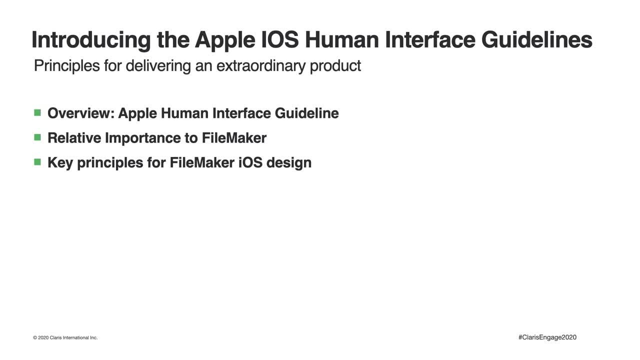 I'll be providing an overview of the Apple Human Interface Guidelines, by no means exhaustive, talking a little bit about how the relative importance of those guidelines are to FileMaker and the key principles for FileMaker iOS design. But first allow me to take you on a little trip. 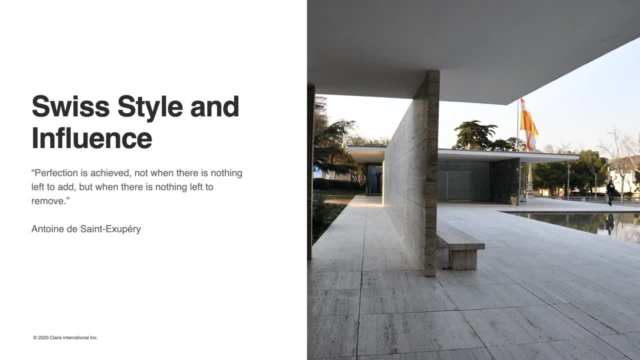 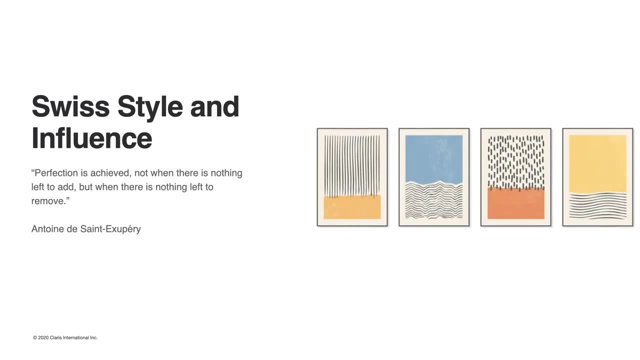 The Swiss style, also known as the international style, emerged from Russia, Netherlands and Switzerland in the 1920s. The design, art and architecture that emerged from this movement, and is still influential today, is the embodiment of an authentic pursuit of simplicity. 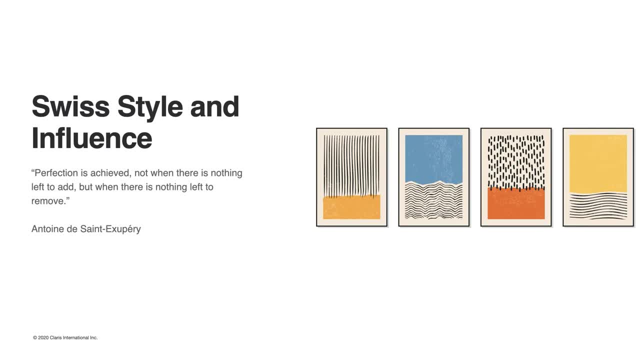 Underscoring that beauty is defined by the purpose, not beauty itself defining the purpose. 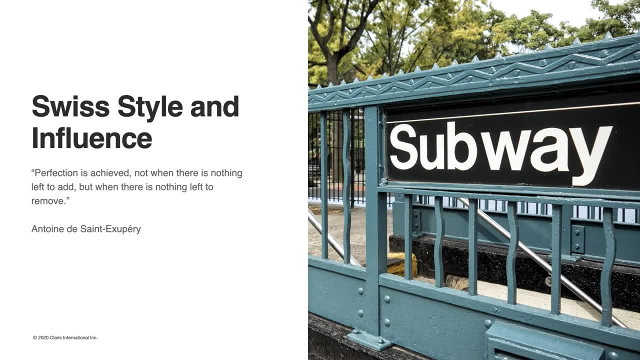 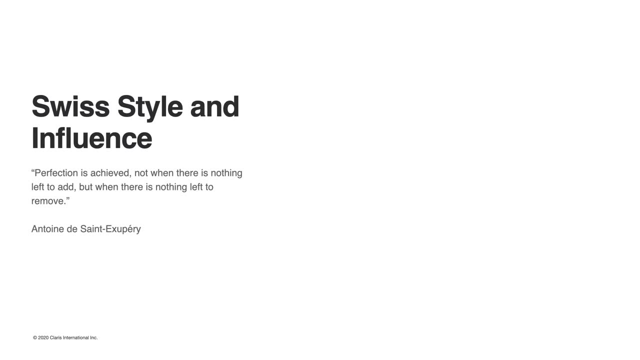 It is an intentional removal of unnecessary elements, leaving a minimalist of functionality behind. Before web and digital, the international style created clean, functional and user-friendly interfaces, primarily in print and architecture, And there were an emphasis on white spaces, the creation of spared panels, the formal 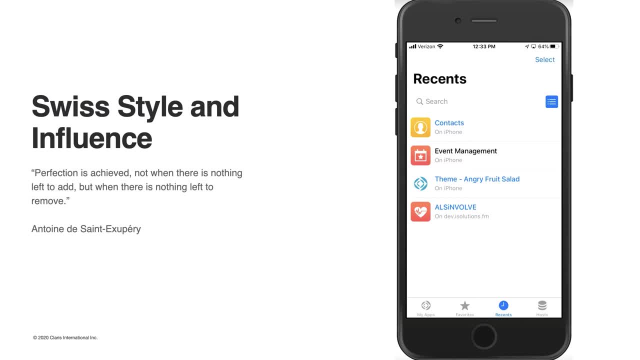 system for applying graphical layouts and grids and superimposed specialCD minerals and and structured information and those that usage of fonts was used to create this unobtrusive method of expression, to give this real, amazing visual impact and establish hierarchy, and it is truly. 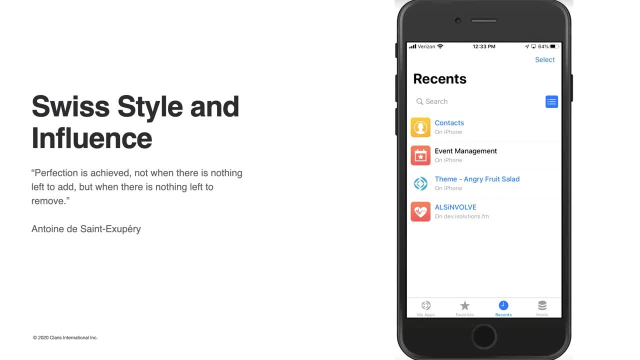 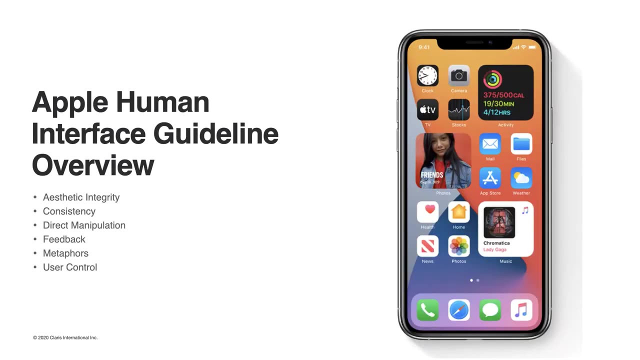 these core concepts that to be understood as to how those those concepts influenced the apple human interface guideline as it is today. the purpose of the human interface guideline is to create a consistent experience across an environment while following key principles it defines. it helps to define how well an app can deliver its function, with meaningful visuals and behavior. it defines 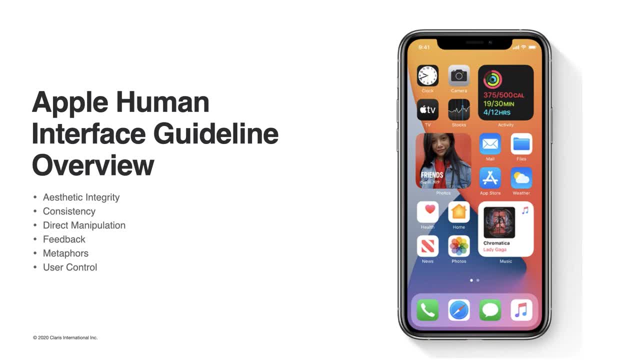 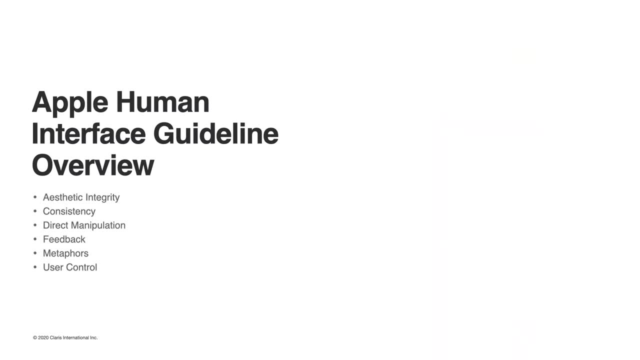 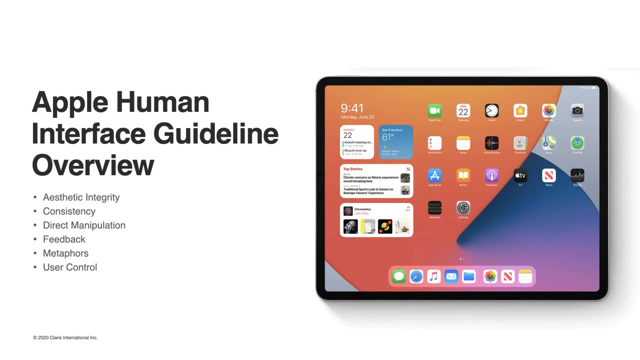 how well an app can deliver its function with meaningful visuals and behavior. it defines how well the app incorporates visual and behavioral familiarity. For example, by using provided interface elements or well-known icons or standard textiles, It reinforces that familiarity to the user. It is the ability to have 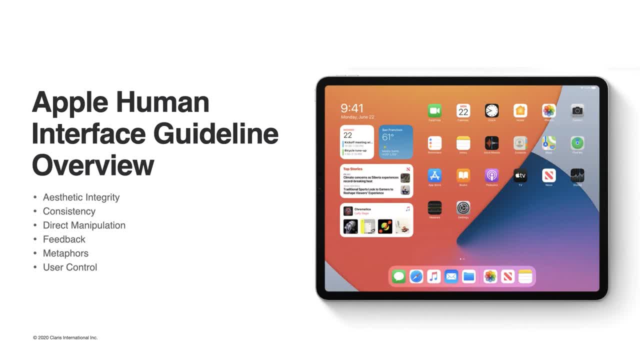 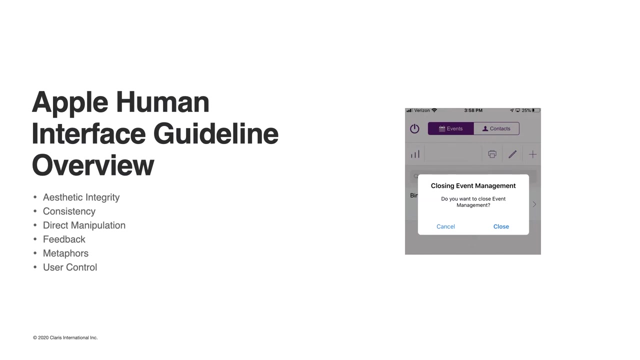 immediate results from user gestures and provide visual, oral and haptic feedback and communication to the user itself. It is using those familiar experiences to provide an intuitive interface for new users, and it also helps us remember that the best experience is the one that the user has. 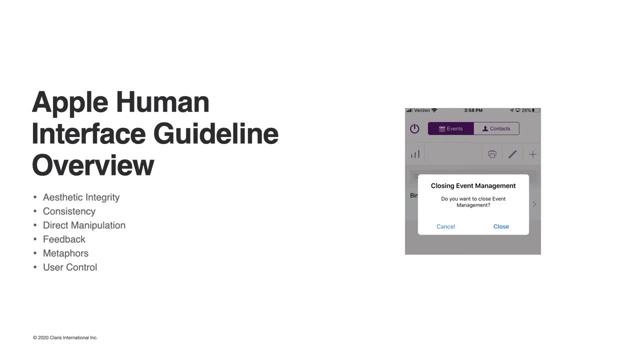 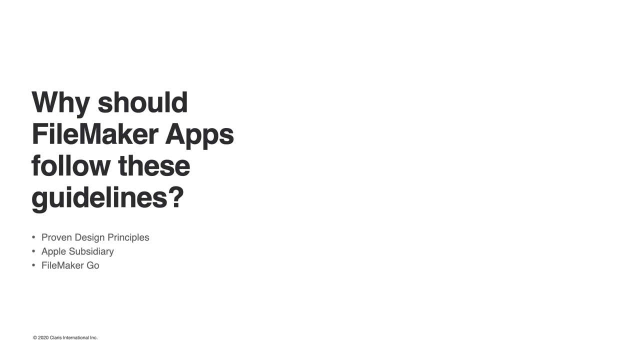 control on the decision-making and the interaction app itself is designed to avoid unwanted outcomes from those user actions. so if we talk about this, why should FileMaker apps follow these guidelines? essentially, we have these proven design principles that will help to create beautiful apps. Claris is a subsidiary of Apple and the FileMaker Go, the FileMaker app itself, is a product of 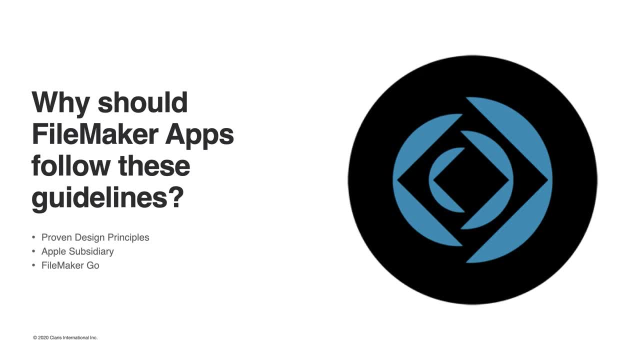 Claris and FileMaker can be, can create apps that are accessible through FileMaker Go, which can be used on an iPhone and an iPad, and it is from that pure understanding of how that app can be delivered that we need to also incorporate those iOS guidelines that Apple has provided in their 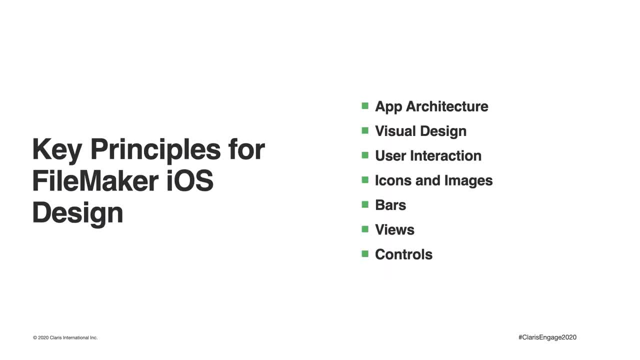 human interface guideline. there are certain key principles that are pertinent that I pulled out for this session. they are by no means exhaustive and for an in-depth review, I would recommend that you take a look at the FileMaker app itself and take a look at the links below if you have any questions, and I'd be glad to help you to process them. 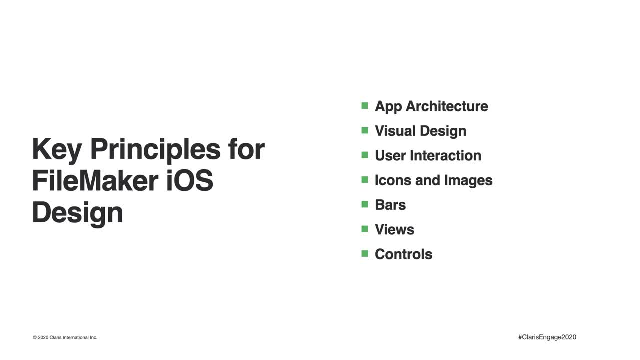 you can also refer to the FileMaker box, and the link to the file that that is available in your home will be there shortly. I would send you directly to the human interface guidelines, the guideline for the. the section on app architecture dives into a very visceral experience of the user from the initial app. 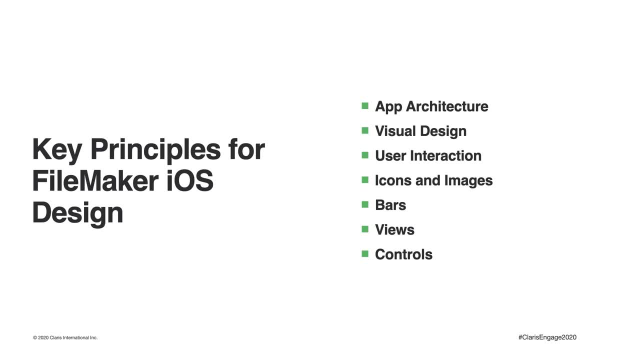 launch to the onboarding process of the user to the app, and thinking about the usage of modals to control where the user is and their contextual relationship to where they will be is something that we will refer to when we are using the FileMaker app in the future as well. 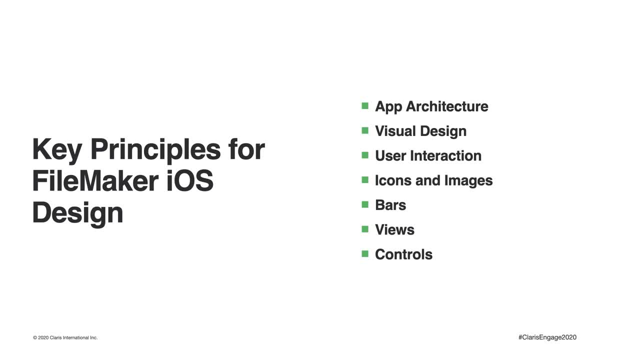 were previously The same with navigation: understanding how to navigate through an application and understanding the different types of navigation that are available. when you're thinking about designing an app, whether it is for a mobile device or for a tablet, And the purpose for considering the design from the aspect of visual design, 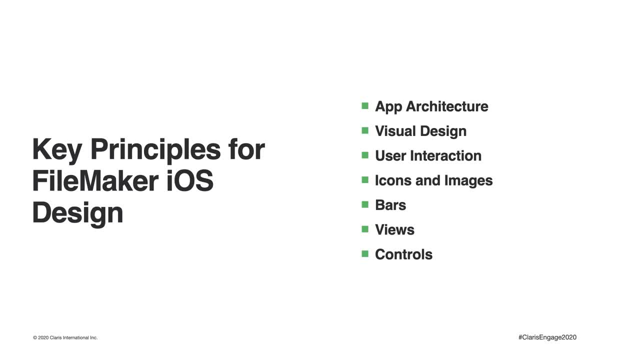 is because we want to avoid confusion of the user. Sorry, not from visual design, but from the app architecture. We're looking at avoiding confusion For visual design. what we'll do is we're actually exploring the principles of creating that great experience. 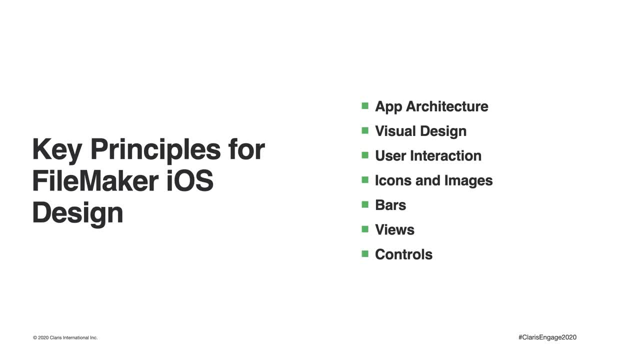 through appearance And, additionally, this principle establishes a commonality through devices And it also establishes a commonality through the use of devices. So if you're also, then goes into a dive into the technical aspect of creating layouts and what areas are margins that you need to avoid and what are safe areas, So that visual design area really covers. 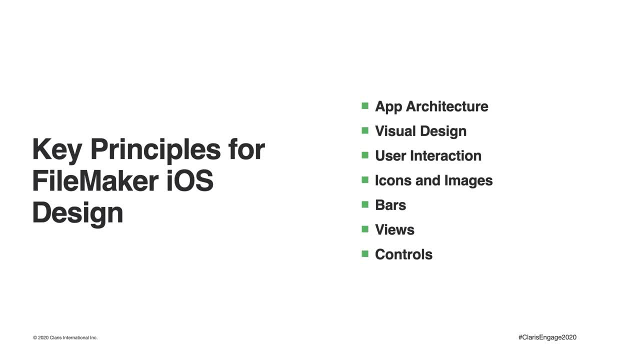 a large swath of principles and guidelines And I'm pulling out, for the purpose of this session, only a couple of those areas. Another section that is important to understand or to even think about is that user interaction section, And, from the perspective of file maker design, the greatest consideration is the 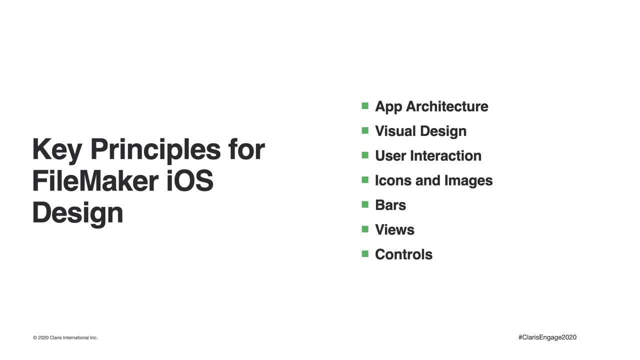 interaction of data entry And from the perspective of the human interface guidelines. what they're really focusing on is the ease of use and speed and usefulness of that data. The bars section of the guideline is thorough in its review of layout, objects and usage considerations of. 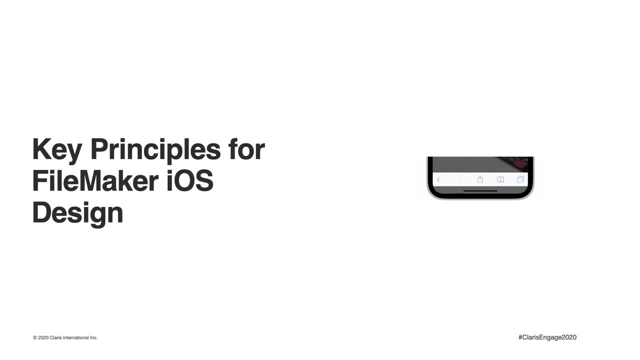 various types of bars, such as navigation and toolbars and search bars, And, for example, while file maker has a robust find mode, there might be layouts where a search mode could be used to provide familiarity, And these guidelines recommend that you go that direction rather than. 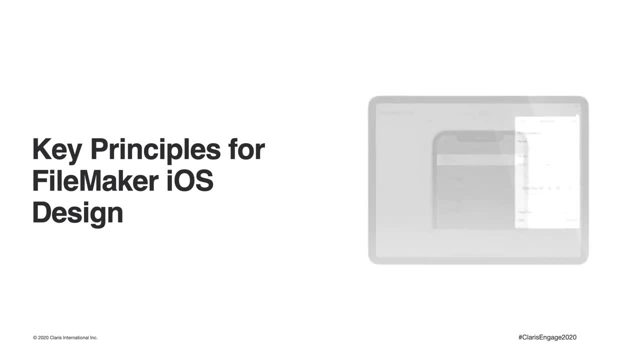 using a text-to-text interface, And so if you're looking for a robust find mode, you're going to have to be very careful about using a text-to-text interface. The views section of the guidelines covers this idea of implementation and behavior popovers. 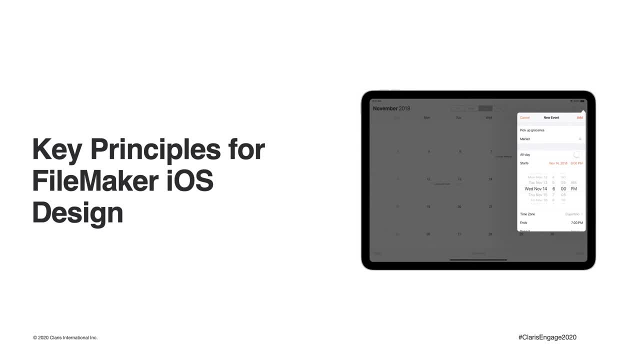 both from a non-modal perspective and a modal perspective, And what I found really interesting about this part of it is that they talked about when and how you would want to consider using popovers, For example. the recommendation is to use a text-to-text interface, And so 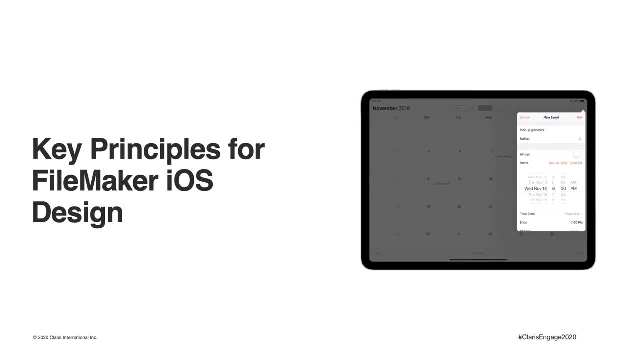 the recommendation is to use a text-to-text interface, And so what they're really focusing is to only use popovers on ipads because you have a larger screen area, and when you're talking about needing some sort of interactive modal or card window or popover for a phone, then what you want 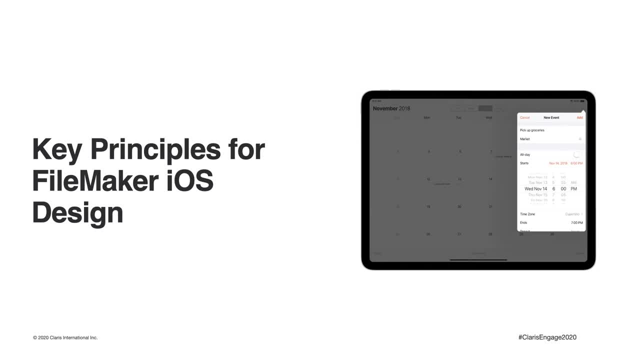 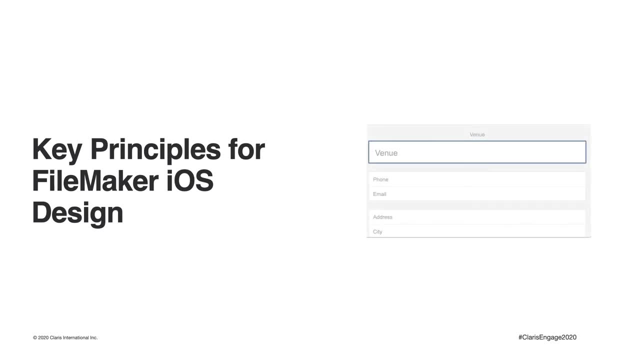 to do is implement a full screen modal in in that case, and the controls encompasses things such as best practices for your layout objects, pickers and labels and text fields and buttons and, where possible, their recommendation to use native ios objects as they are available, because this creates 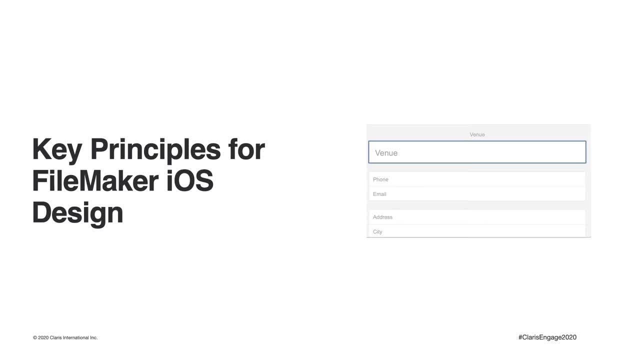 a consistency and familiarity for users, which is really the sort of the. this is one of the key points of the takeaways from the guidelines- is creating consistency and familiarity. you, for example, text fields they. the recommendation is that we should put in hint text to just let. 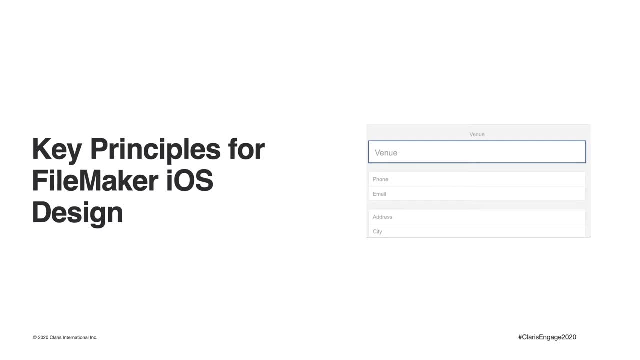 the user know what type of data or what what thing is being expected to be entered in that field. that way you can you can start to save room on on layout objects so that you're not having the labels are inside the field and not above the field. it creates a clean look and it also 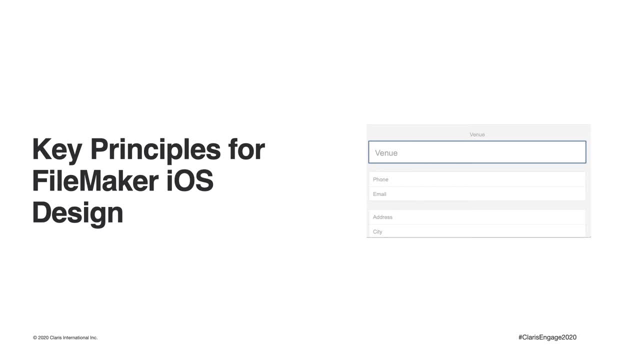 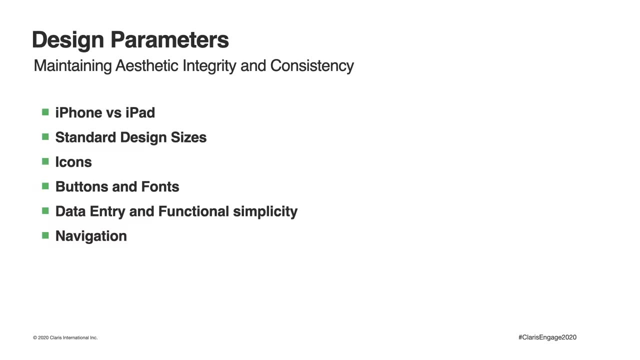 eliminates the fact that the labels are inside the field and not above the field, and that eliminates the need for redundancy. in this chapter, we'll be going over design parameters that are used to be able to maintain that consistency and the aesthetic integrity of the app that's being designed, and in this case, 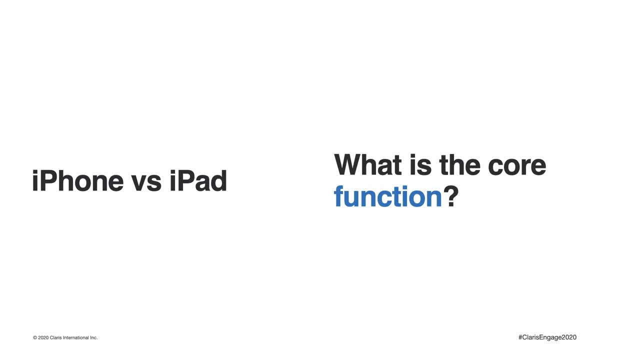 it's our file maker app. the first thing that we want to think about when we are talking about the design of a mobile app or an app for a device is: what is the device that you are going to be using and what's really at the core of it? what's, what's the function that you're trying to achieve with? 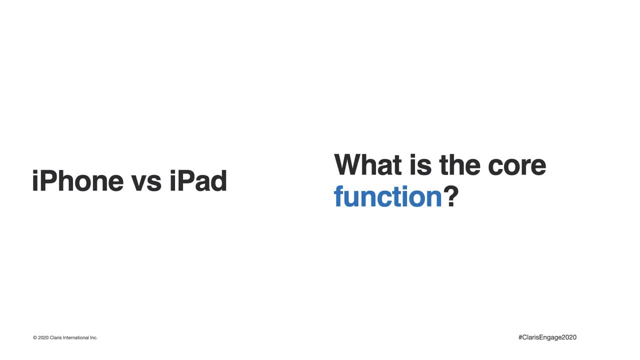 that device. so does your function. is it appropriate for that function to be used on an iphone, or is it appropriate, or is it more appropriate to design it for the ipad? and by asking questions you will come up with the answer for that. so that's the first thing that we're going to be talking about. 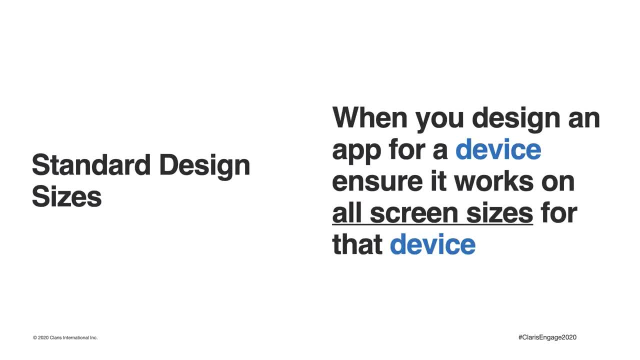 once you have decide upon your device or devices that you will be designing your app- or potentially multiple apps, smaller functions within a single app- then what you want to do is you will need to design for the device that you have selected. so if you have selected a, an app for the iphone, then 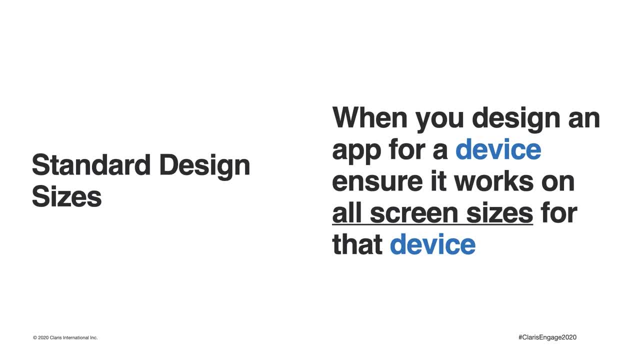 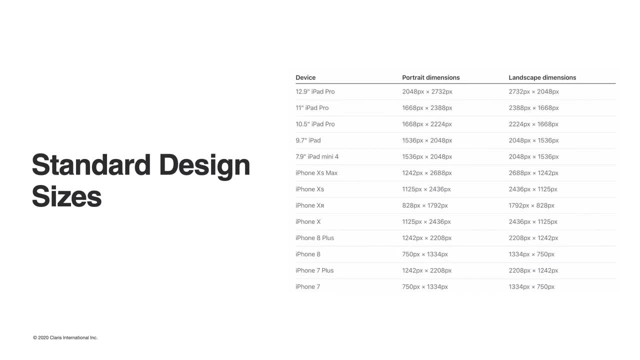 you will also need to be able to design your layouts so that they will work on all screen sizes for the iPhone. Luckily for us, the Apple human interface guidelines has already given us the table that shows us what those, what those basic resolutions are, the dimensions for those devices, and so you 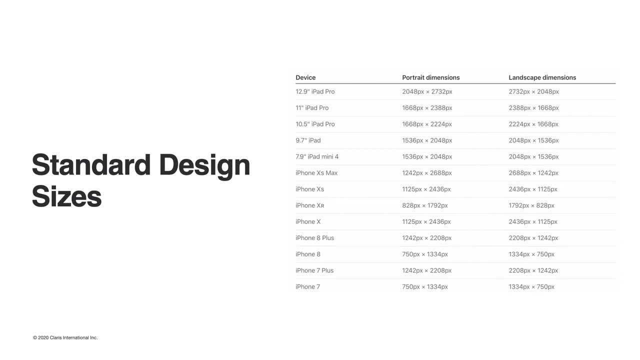 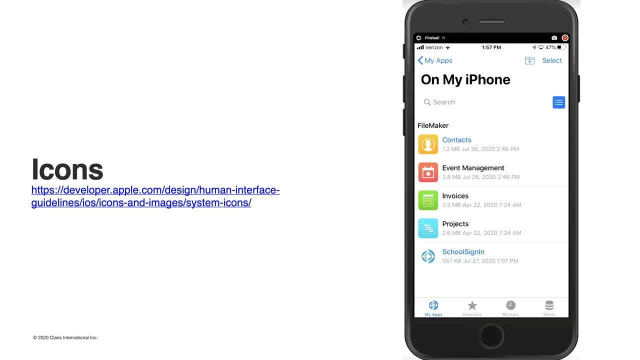 can go to there and find out what the dimensions are for portrait and for landscape, and then that is the beginning of your design sizes there for icons. one of the things that I found very interesting with the, with the human interface guidelines, is this idea of your custom app and the importance of 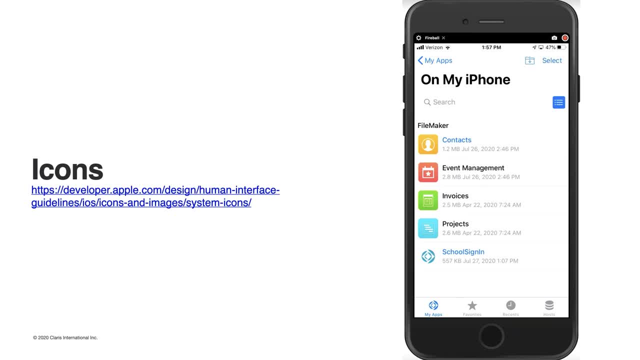 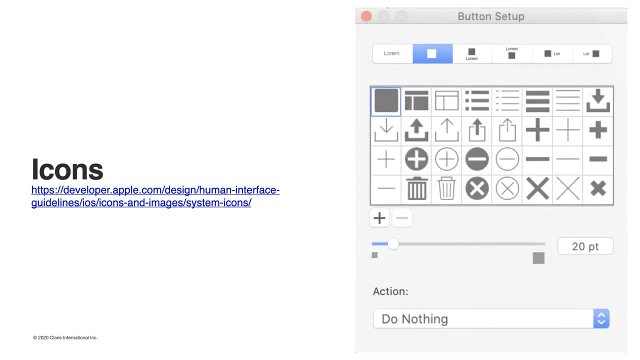 that custom app it is. it's the diff, it's the defining icon for that app. so it's what you see when you go into the FileMaker Go menu and then you are doing your design sizes. So that's why the design frame is so empty. 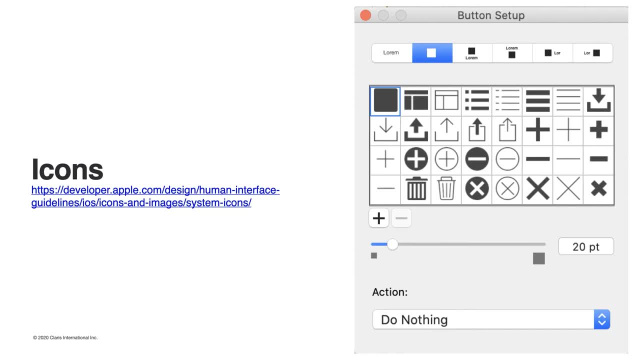 but I'm going to do some more stuff in a few minutes. It'll allow you to find that app immediately because you're familiar with that icon for it. The other section that I found very interesting on icons was this idea of using native icons. 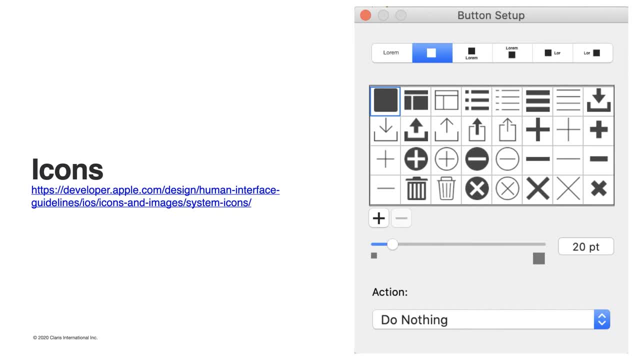 And then when do you want to consider creating a custom icon? Because the thing that you really need to do is establish your consistency with your icons. But it's not just your app, it's all the apps. So Apple has created, within their guidelines, a section of that where you can go and see all of the icons that are there. 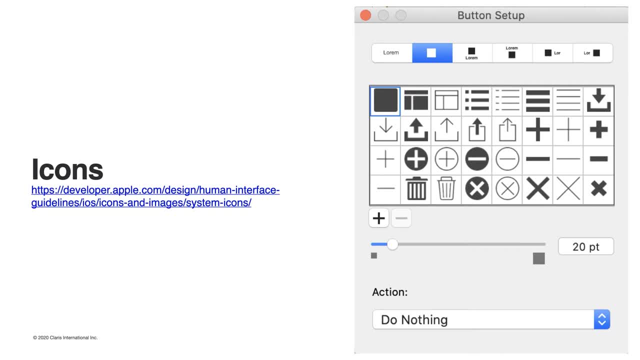 and the meanings that are related. So, in order to avoid confusing users, it is truly essential that we use the images for the meanings in which they were intended. So it would be better for someone to decide that they need to create a custom icon because there isn't an icon that exactly. 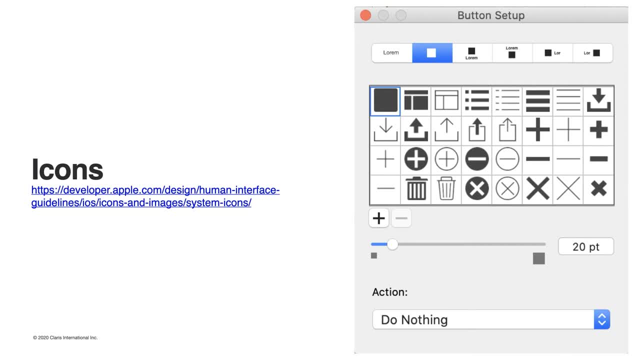 means what they are trying to portray with the usage of that icon. So if you've got something that's close but it's not an exact meaning or not an exact match for your meaning, it is better to actually create your custom icon rather than co-opting one that exists and then creating confusion later for users. 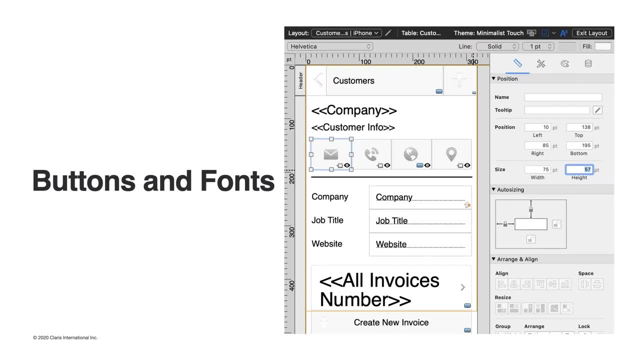 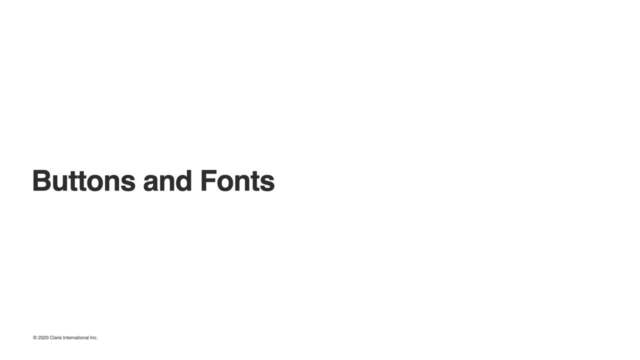 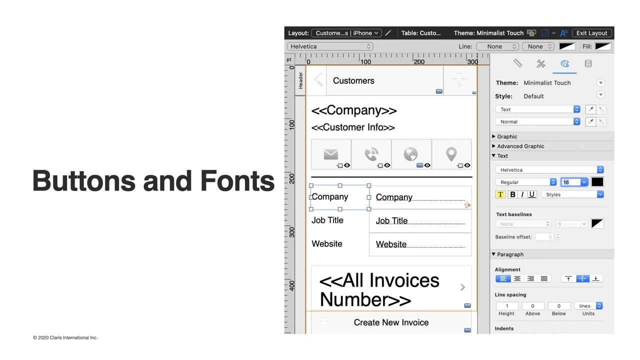 Another aspect of the human interface is that it allows you to create a custom icon. So I want to say that the most important aspect of the human interface guidelines is the sizing and usage of buttons and fonts. I would recommend that, if you need references for these, that you go to the FileMaker starter apps and go to the ones that have iPhone and iPad layouts. 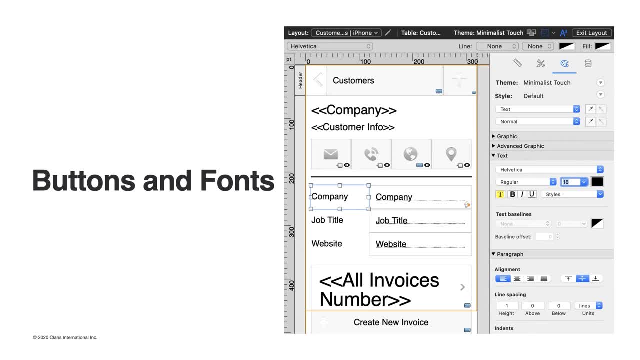 because those have the buttons at the minimum sizing. It has the labels, It has the buttons, It has the tools with their minimum sizing for the text and the fields with the minimum size, the minimum height for the display of those fonts. The only other things that you want to consider when you're thinking about the usage of buttons. 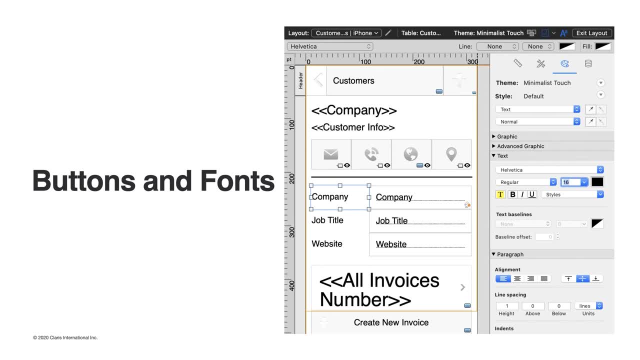 is that when buttons do spread across the screen, so if you take them across the bottom of the screen of an iPhone, you want to avoid stretching that button across what are considered the margins of the phone, So instead it would be better to keep the button within the constraints of the safe area. 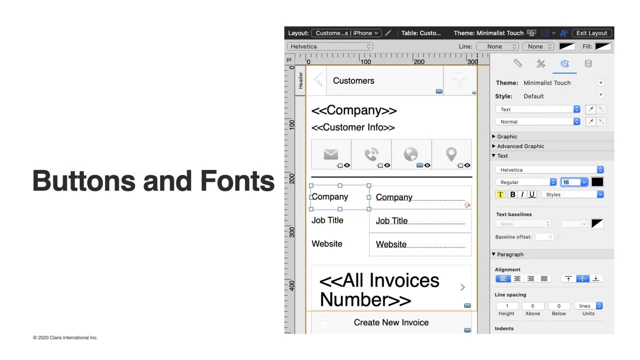 and then curve the corners of that button. But truly it's best to go ahead and do that. It's best to go ahead and look at the starter solutions, because there's no reason to recreate the wheel. They have them there if you need to understand. 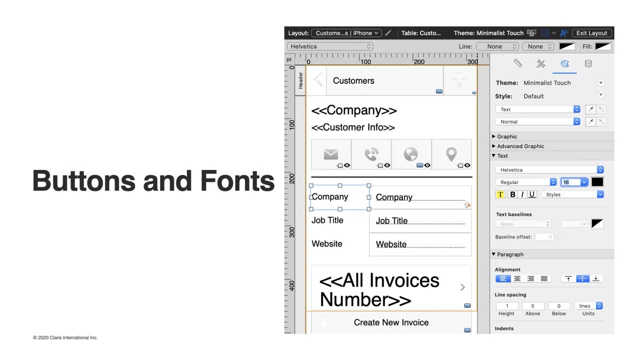 oh, I need to remember that my buttons are 44 pixels in width and height. then you can go there and you can confirm it. It's a very easy way to just make sure that you're designing to the proper sizing for a mobile device, for a touch device. 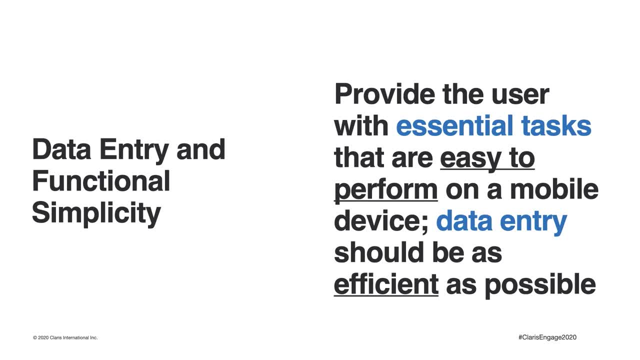 When we talk about data entry and functional simplicity, what we want to do is make the idea of data entry as efficient as possible, And we want to give the user the ability to have essential tasks that are easy to perform. So we don't want to make things complicated. 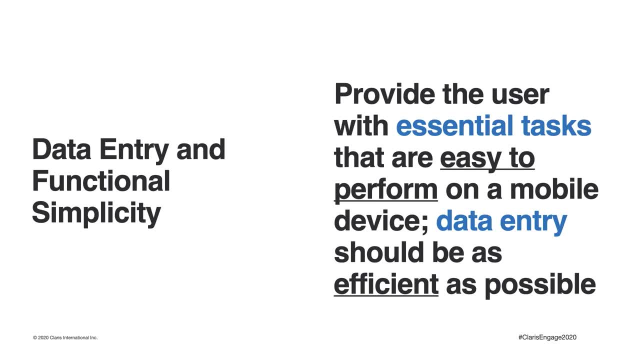 and we don't want to ask the user to do more than they need to do to do the thing that they are being asked to do on that device. For example, you might consider using a picker or a table instead of a text field to choose from a list of predefined options. 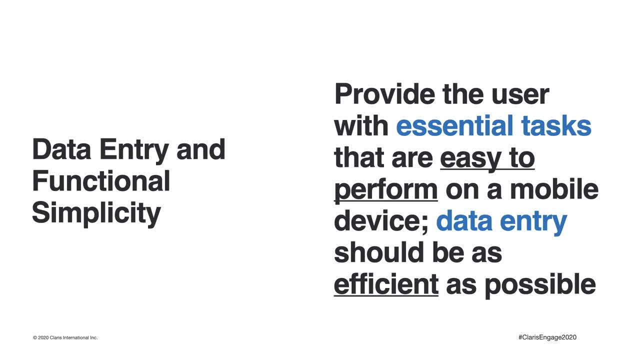 Rather than typing in something into a field, The other thing that might be considered is using data that's been previously entered, so that the user doesn't have to enter that information again. One of the things that FileMaker can do quite well is to validate field values. 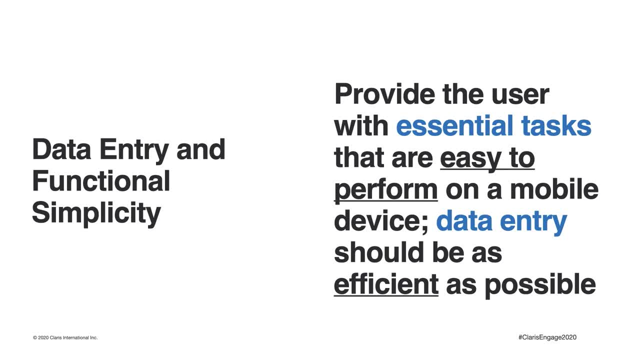 So we know that we can do field validation really easily. That is definitely something that is a recommendation within the guidelines themselves. The other part of it is, then, to don't make every field required, but only make the fields required that are necessary, Because, again, we're balancing this idea of allowing the user to do their job. 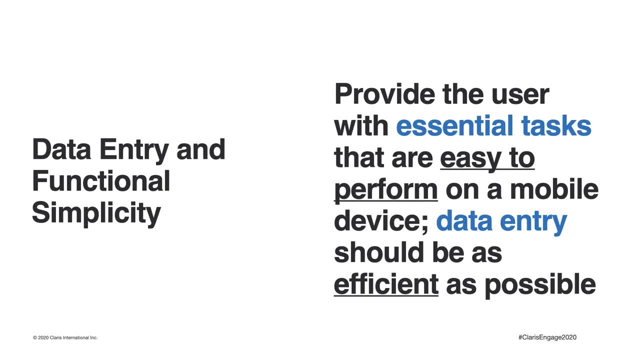 but also not making it too difficult on them to do what they need to do, And we've talked about this before. but one of the other things that could be useful for a user is, instead of having layout labels, text labels on every field that we use, the hint text inside the field itself. 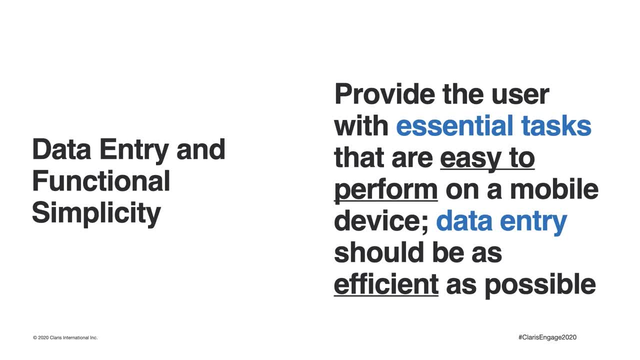 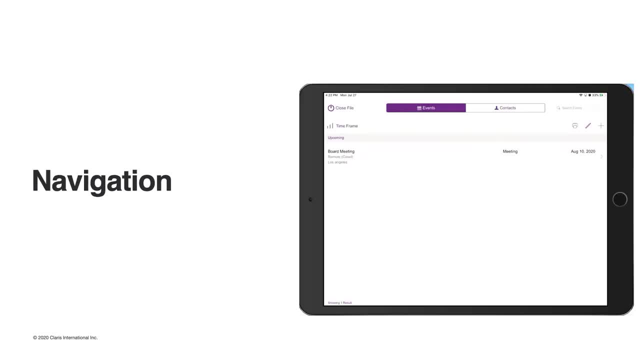 that gives the user some additional white space to ease the visual impact of the app on them. Navigation should feel natural and familiar and it really shouldn't dominate the interface or draw focus away from the content or what you are or the app, the purpose of the app itself. 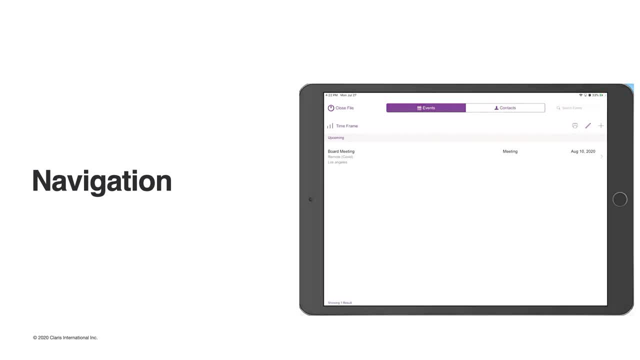 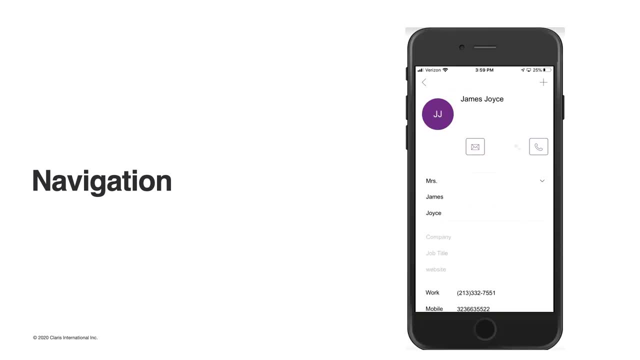 And so users are definitely familiar with the back button and they'll know how to use it to go back to their layout. So go ahead and use a back button when you want to bring somebody home. Button and tab navigation are a great way to. it's a very natural way to navigate through an app. 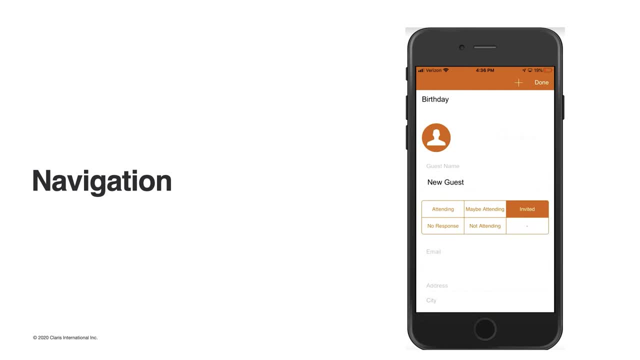 but you want to also then be careful that you don't leave your users trying to figure out how they're going to get back And in the case of like, let's say, entering a new record, you could have that done button that returns them back to their previous layout. 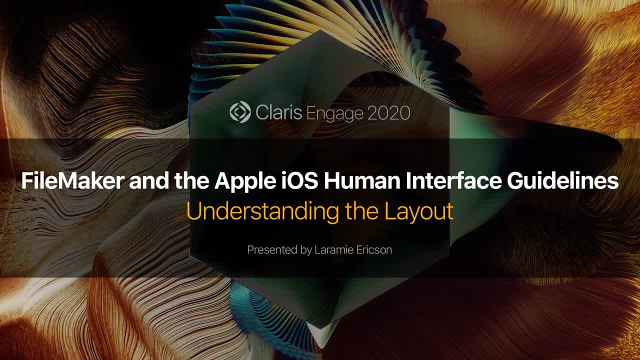 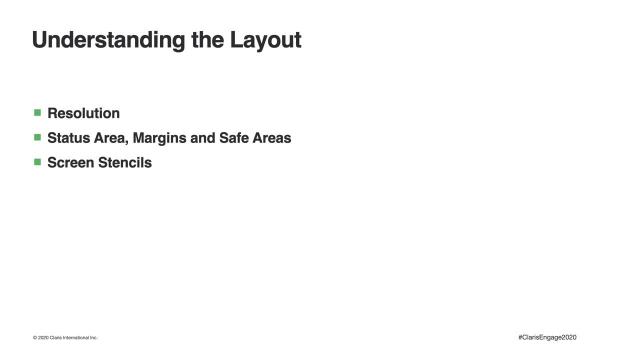 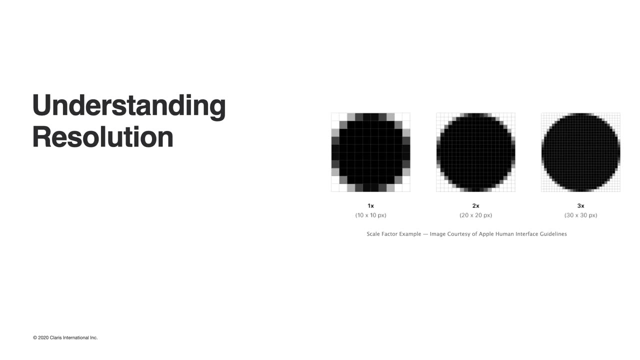 This next chapter is all about understanding the layout and how to understand the sizing and resolution on that layout and how that impacts the objects on your layout. So when we think about understanding resolution, what we need to understand is that with a standard screen resolution like a desktop screen, 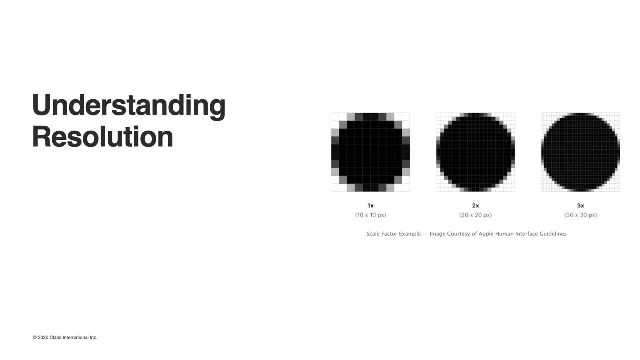 the ratio, at least today, is one point to one pixel, And as you move to devices that have higher resolution or that use a retina display, what you see is an increased number of pixels per point on the screen, So something might be the same size in one area. 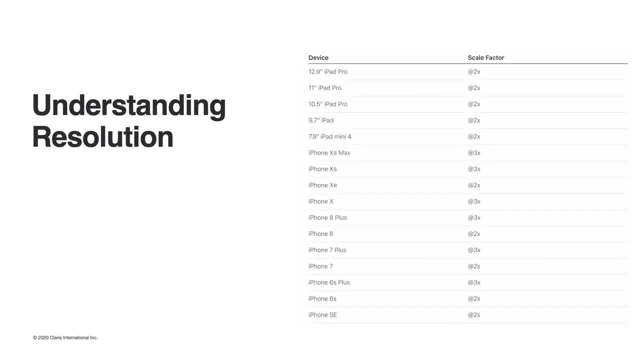 will look much smaller on a device that has a higher resolution. So if you want to have that object look appropriate based off of the resolution, then you need to increase the size of that object. The other thing to consider here is this idea of scale factor. 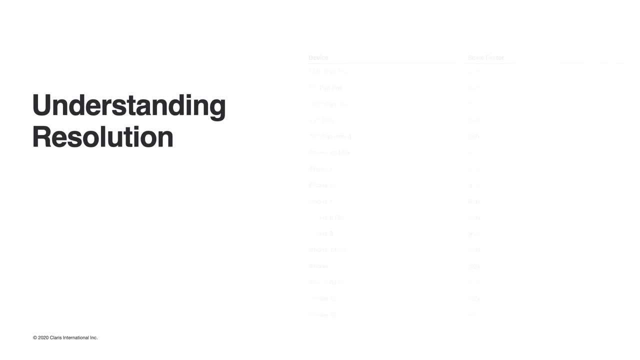 And scale factor is essentially predetermined by the objects themselves, by the devices, And it's available both in a chart form on the Apple Human Interface Guidelines and also if you go to one of Matt Piotrowski's theme files. he has them laid out on the devices themselves. 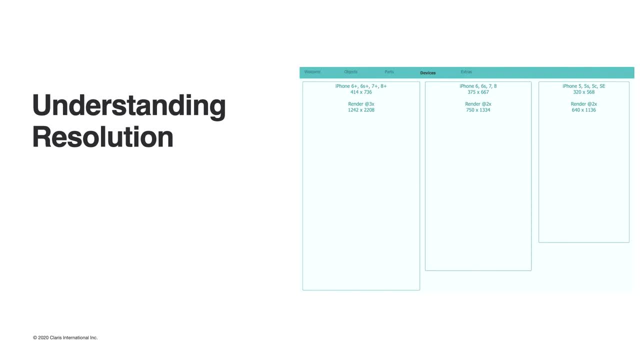 So he has a tab and it shows you like: here's your layout, here's your usable area of your layout, And then he also indicates: what does that render? what does that scale factor do? So what do you need to multiply by to be able to make things look appropriate on that device? 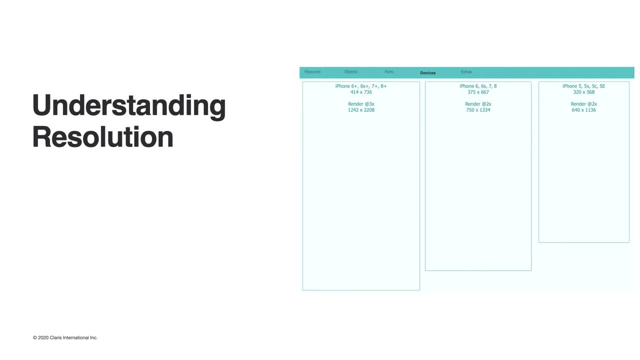 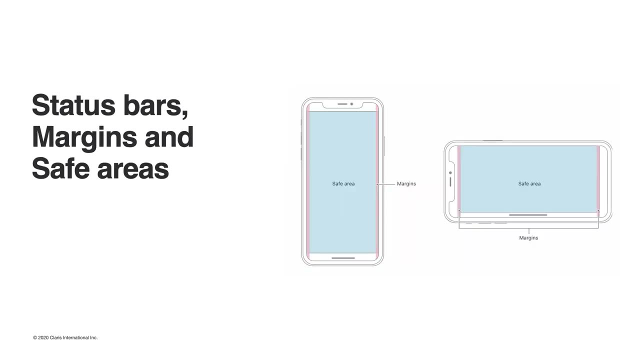 And it changes per device and you can go reference that within the interface guidelines themselves. The other area that is useful to consider is this idea of what is a safe area and what is a layout margin, Because, while the iOS UI Kit provides those margins to developers, 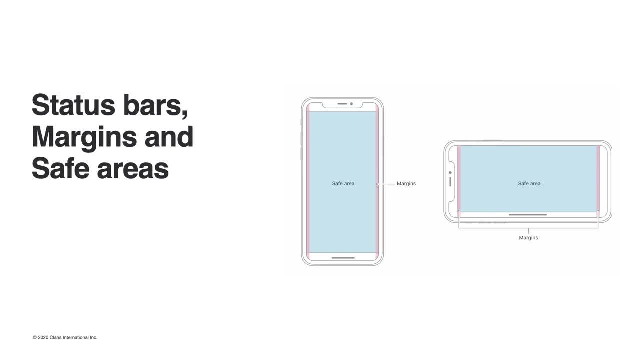 in FileMaker. we don't have the constraint, we don't have any constraints of those margins. Even if we create a screen stencil, there's no constraint to go outside of those margins. So we need to be aware, when we're designing an application, of where do those areas occur. 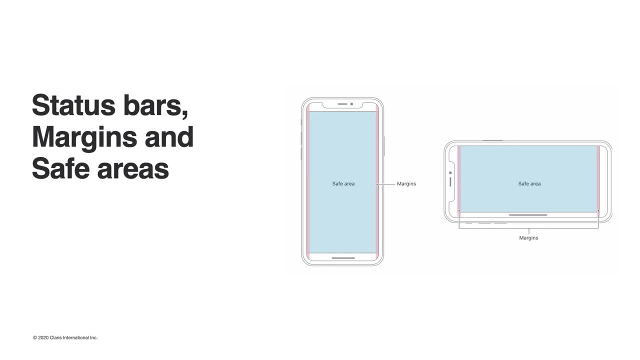 and how do we avoid them. So, for example, the status bar appears at the top of the screen, except on the iPhone in landscape mode. So if you're designing for landscape mode on an iPhone, then you don't need to worry about the status bar. 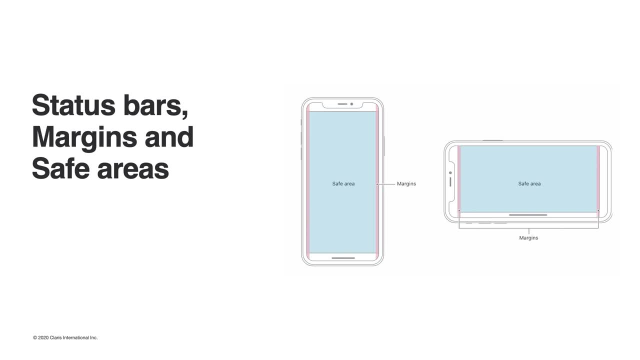 But in other cases you do need to know that that is going to appear there because it's part of the iOS. And the other thing to consider is gestures. So because gestures are used commonly on touch devices, the margins of the device should be left free. 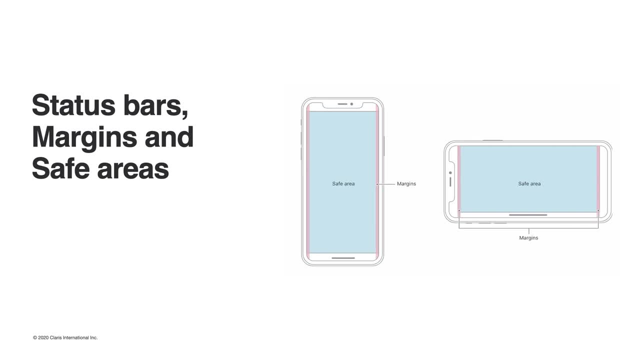 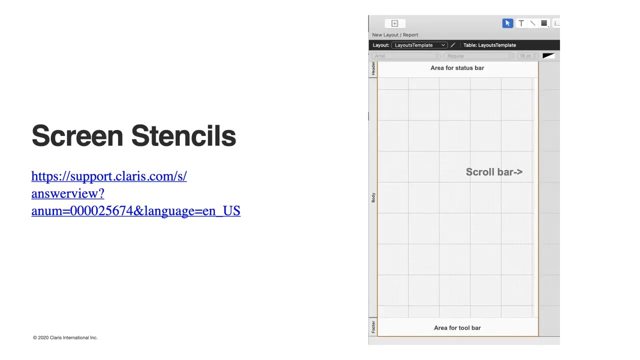 of any functional objects, such as buttons or data entry. So those are your in the image. here it's the red lines that are on the sides of the device. The screen stencils are incredibly useful for being able to define your usable space. 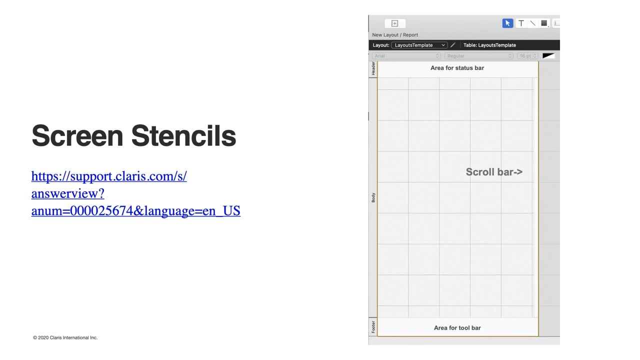 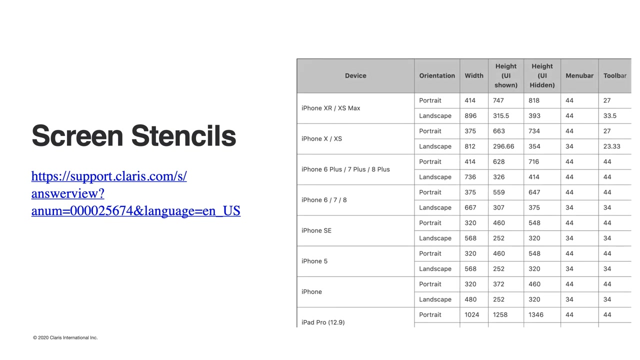 And it's useful for avoiding this left to right scrolling when you're looking at a device, especially a design that's put on a mobile device. However, what the screen stencil doesn't prevent is your layout objects going over or past the stencil itself. So, FileMaker- sorry, Claris- has an article. 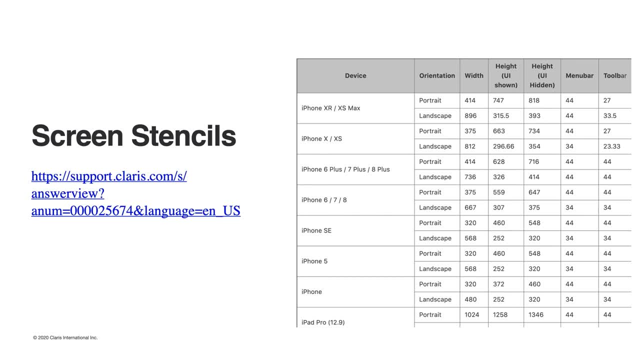 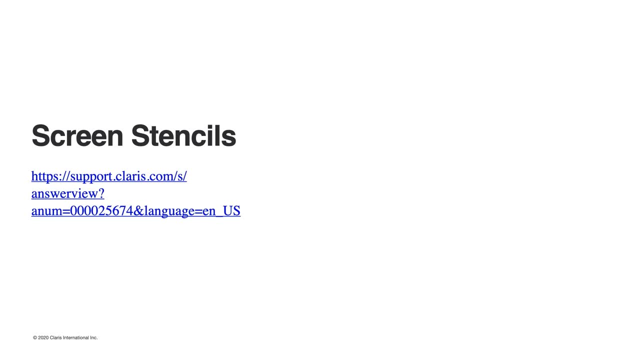 where they define what the usable space is and then what parts of that usable space are taken up by the native menu bar and the native toolbar for FileMaker, And then you can- so it's useful- to create some sort of either a screen stencil or just take a rectangle. 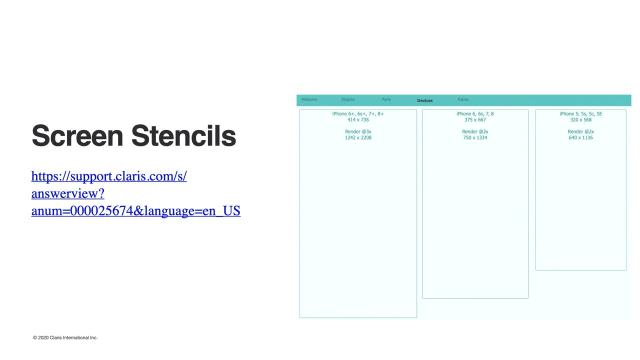 and put it in there, of what are those areas. So then, when you're drawing, when you're applying your design, you know that you're not going past those usable areas and you're not creating unwanted areas or unwanted or undesirable effects on your, within your app, on your device. 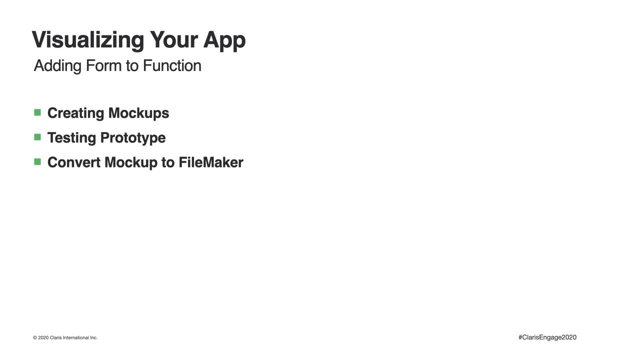 In this chapter. what we're going to do is take all of the information that we've used from understanding what the guidelines are and applying them to the actual visualization of the app design itself. So the first thing that we'll do is we will 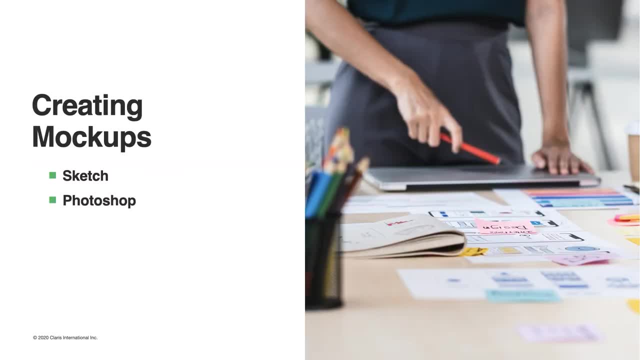 you'll begin to create your mockups, And mockups can be done in a number of different applications. There's Sketch and Photoshop, Adobe XD. There's also Lucidchart, Drawio, MyBalsamiq, among many others. 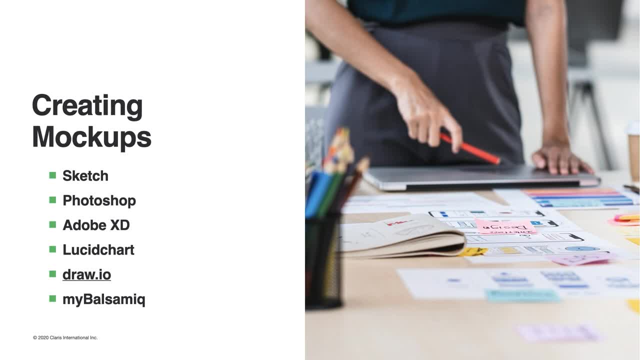 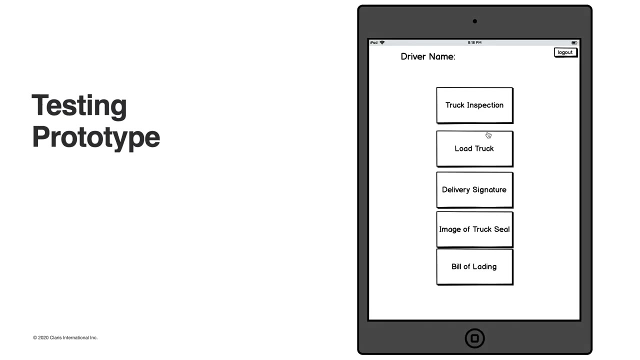 So once and then, once you have gotten your mockups to the point of where you feel that they are ready to be ready to be transferred into a prototype, then one of the things that I have found very useful to do is to take a pro, take a PDF of that. 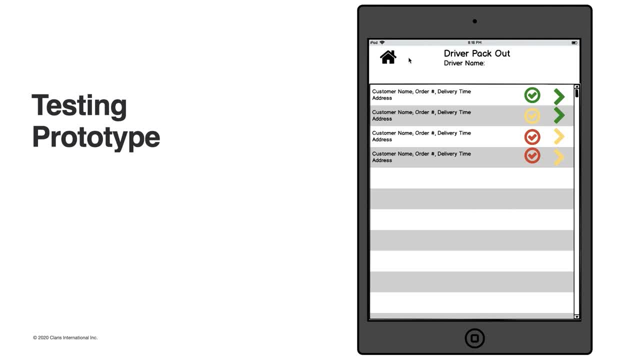 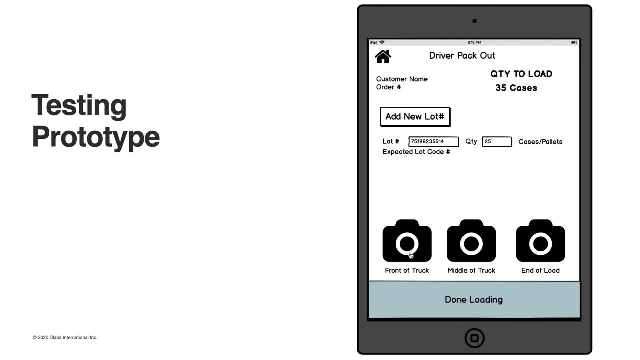 and then create a movie on the iPad or somewhere where you're actually observing the users, looking at where they're clicking, looking for hotspots, seeing if there's anything that needs to be changed about the mockups itself as you're working your way into your prototype. 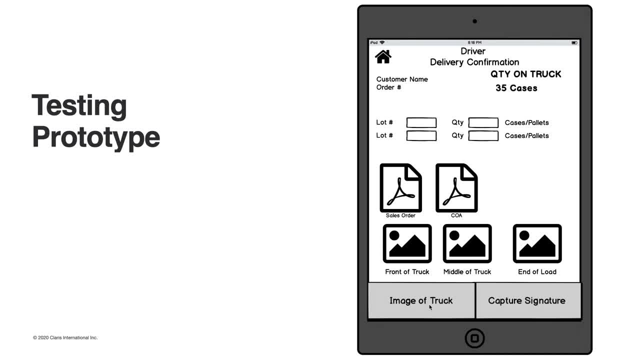 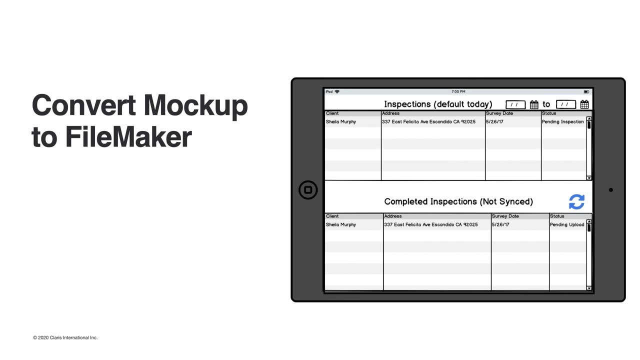 It's also a great way to be able to just take a look at touch sizes: Are your fonts large enough? Are your buttons large enough? So, and then, once you have gotten your app to the point at which you are, once your prototype is working. 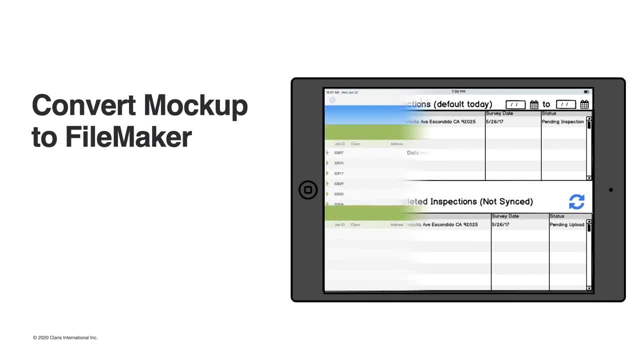 and you are ready to build in FileMaker, then you can take your prototype and your mockups and convert them into your FileMaker application, Don't? I wouldn't be concerned if things change a little bit, going from mockup to prototype to application. 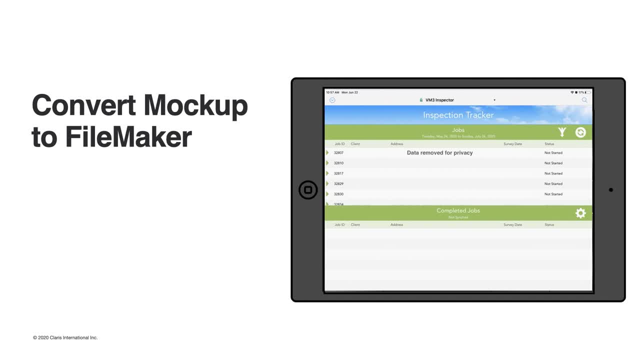 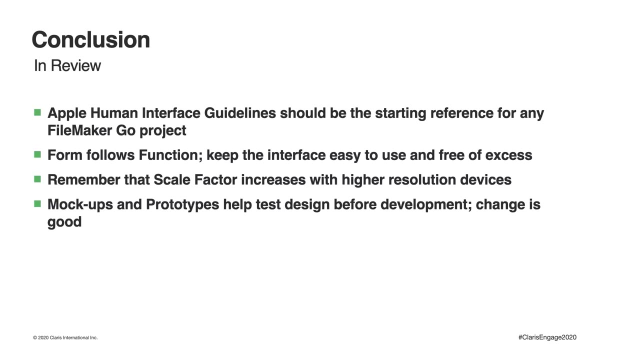 because as you go through each one of those steps, you're going to find out something different, and change is totally appropriate and it's acceptable and expected. In conclusion, there are a few points that are good for takeaways on this. One is that the Apple Human Interface Guidelines. 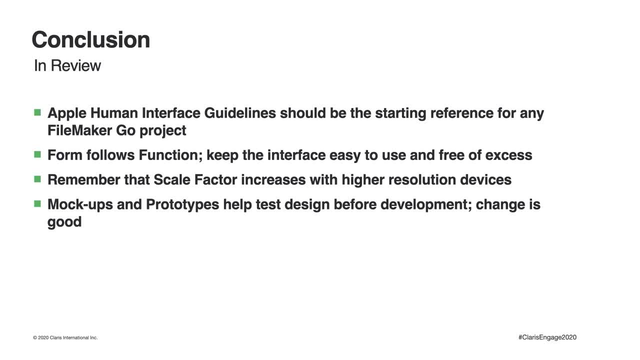 are a great reference to start before you begin to plan a FileMaker Go project. Remember that form will follow function. You want to keep things simple, So keep your. keep the simplicity, make the interface easy to use and avoid adding in extra things to it. 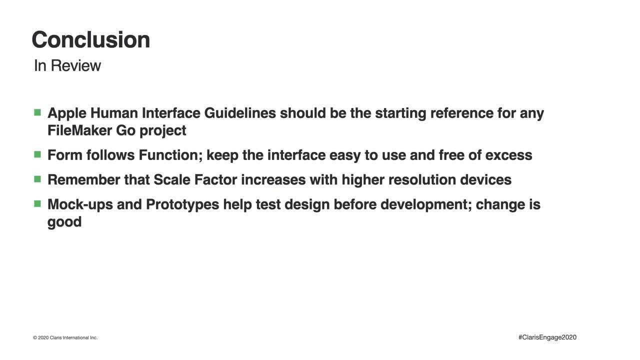 Remember that the tip about the scale factor, that it the scale factor increases when you get higher resolution devices, but on the screen itself your objects will look smaller if they haven't been scaled up to match for the scale factor, The scale factor of that device. 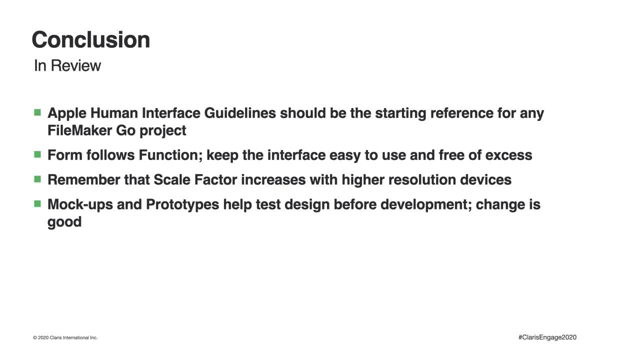 Some of the app, some of the mockup apps that are out there, will actually convert a mockup to the scale factor of the device, So that Sketch has that and Adobe XD has it and Photoshop has it. I don't believe that the others do. 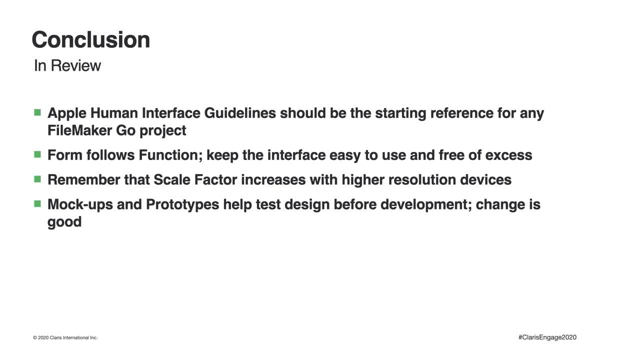 And for our mockups and our prototypes. they can help you test before development. And also don't don't don't worry if things change, because they are intended to change every, every iterative step that you take from mockups to prototypes, to development. 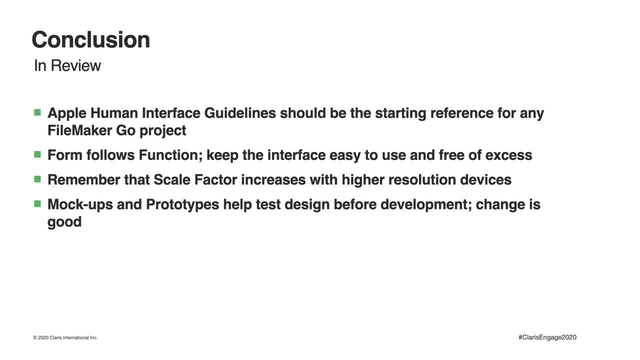 You're getting some iterative changes that will improve, improve the app itself And if you refer back to those interface guidelines, you'll always find great little snippets of information that might be useful for you. at that time I used quite a number of references. 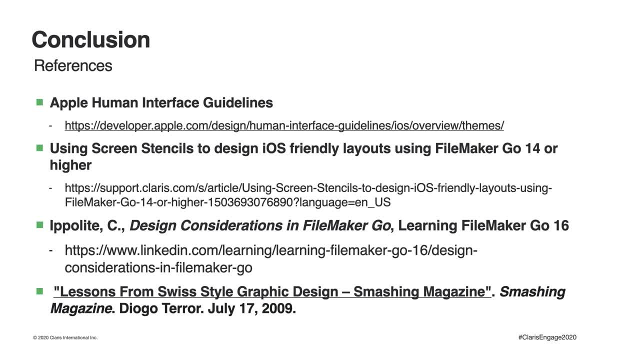 to put together the materials for this session. First and foremost are the Apple Human Interface Guidelines themselves. Claris has a great article on the usage of screen stencils, And then Chris Ippolite in his design considerations for FileMaker Go. he was really the influence. 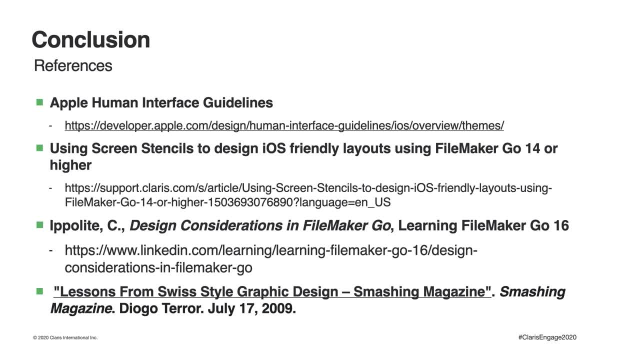 of me to just kind of go like I need to. I need to remember to go back to those starter solutions because those are- they actually have really good information inside of them already and no need to reproduce the wheel on it- And for information about the international style. 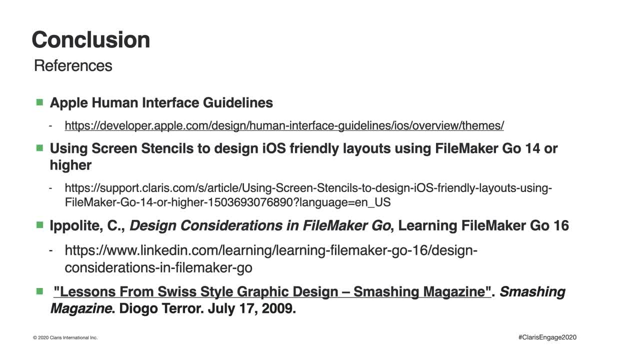 was this article from Smashing Magazine. There's a number of other articles out there that talk about the influence of modern design, modern graphic design, from the international style.